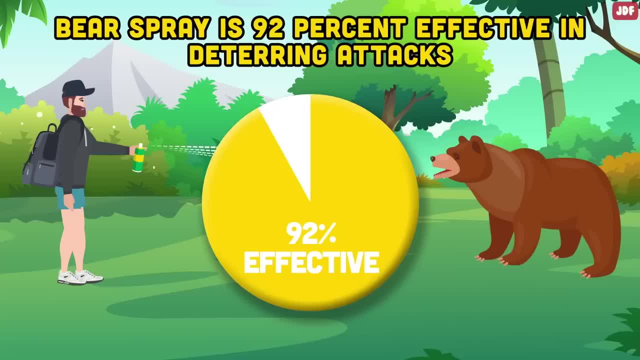 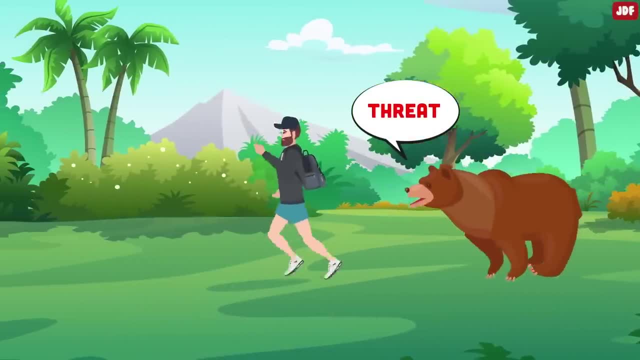 Research has shown that bear spray is 92% effective in deterring attacks from these animals. If you don't have a bear spray and you end up on a date with a grizzly bear, play dead. Grizzlies will stop attacking when they feel you are no longer a threat. 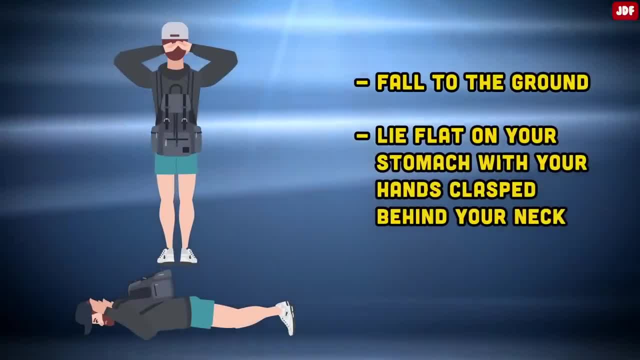 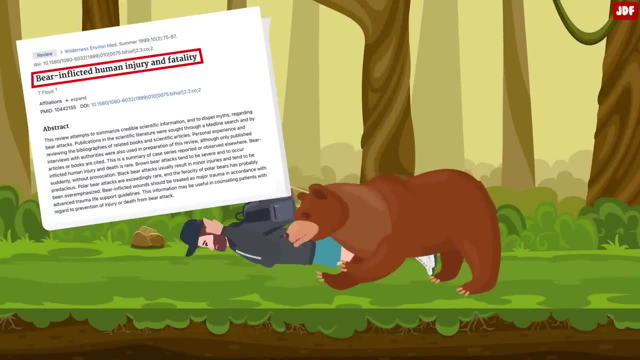 Fall to the ground. lay flat on your stomach with your hands clasped behind your neck. Spread your legs to make it harder for the bear to turn you over. According to a study, the bear is likely to survive the attack if the victim can lay still, even if he is playing dead. 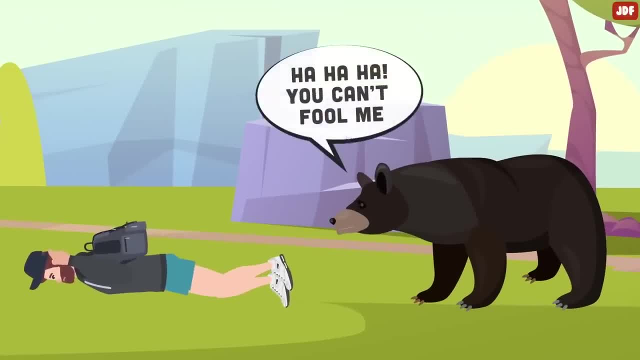 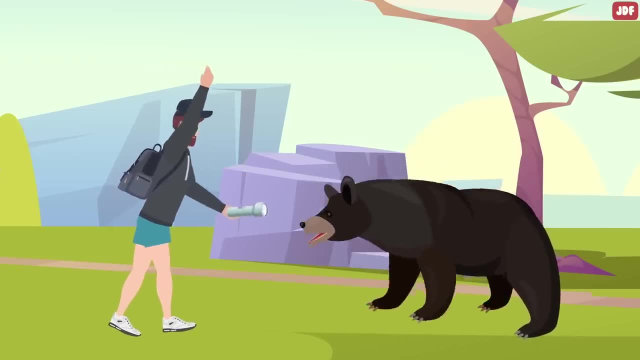 With black bears, though, it's different. Don't try to play dead. They don't fall for that. Your best bet is to make yourself look big and fight back using any object available. Concentrate your kicks and blows on the bear's face and muzzle, And don't try to climb a tree. 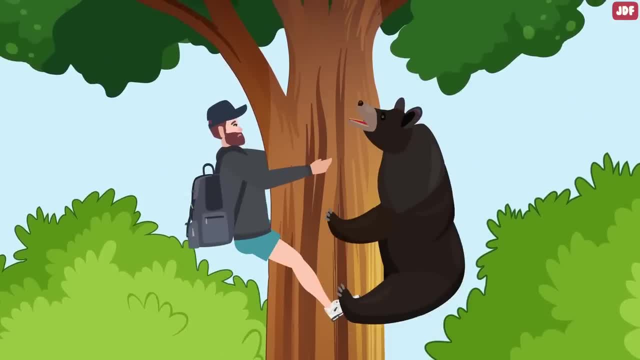 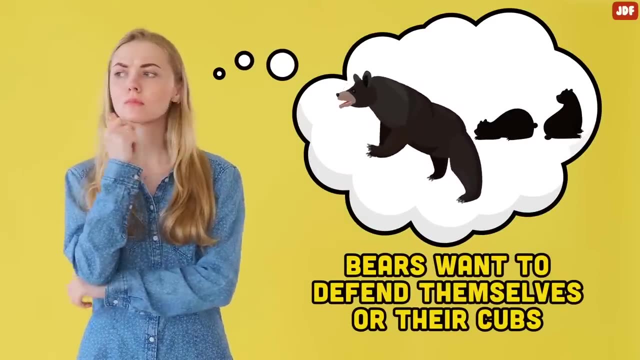 since both black and grizzly bears can climb that tree faster than you can. It's important to remember that, while most bear attacks occur because the bears want to defend themselves or their cubs, there are times that they attack to hunt you. Pretty much all scientific. 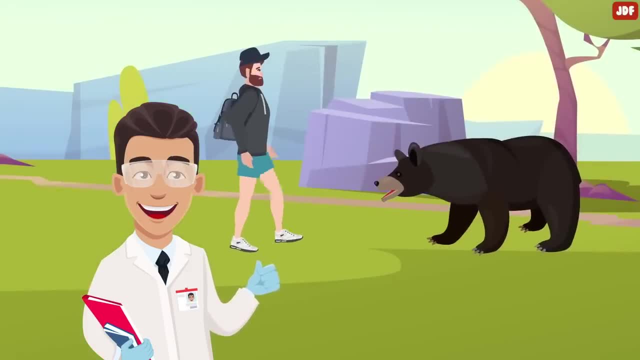 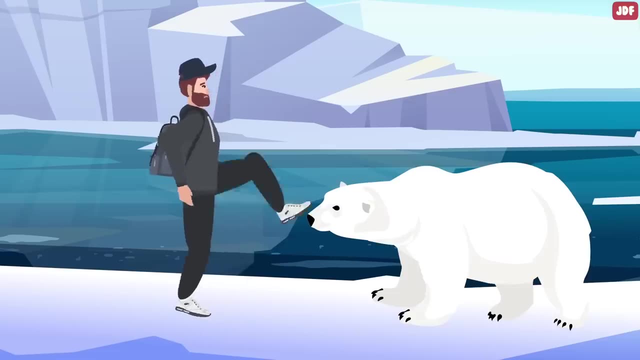 guides agree that if the bear sees you as food, you should fight. This is often the case with polar bears. To a polar bear, you're a prey at first sight. Strike back by aiming for the nose or eyes And don't play dead Snakes. 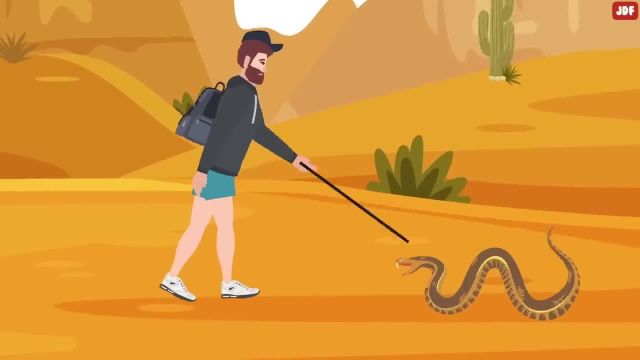 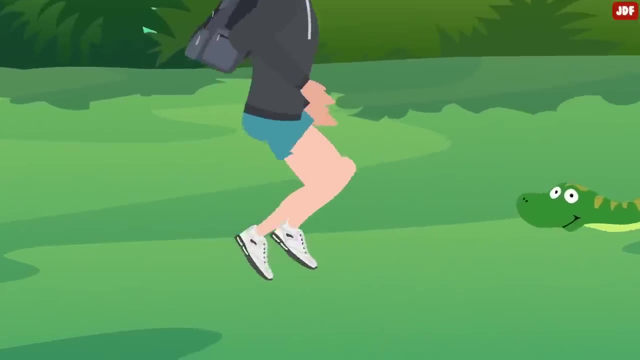 Most snakes are neither venomous nor dangerous. These creatures don't generally attack unless provoked, so it's best to leave them be. If you notice a snake is following you, stomp your feet hard on the ground. Although the snake will not hear, the noise, the vibrations the stomping makes will scare it off. 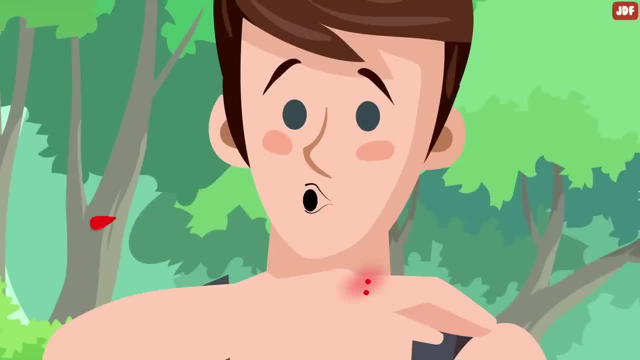 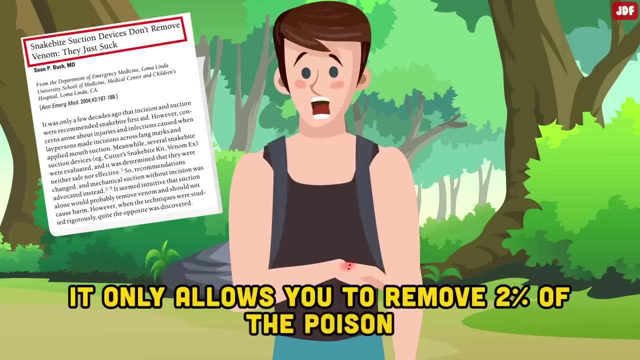 If you do get bit, don't try to suck the venom out of the wound, as they show in movies. Research has shown that this method isn't effective. It only allows you to remove two percent of the poison. Even worse if you have an open wound in your mouth. 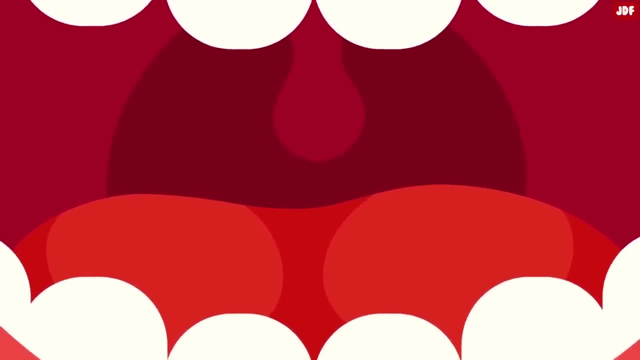 the venom could spread into your mouth. If you don't do this, the venom could spread in your bloodstream even faster. And don't apply tourniquet to stop the poison from spreading. Studies suggest that applying a tourniquet does nothing to help the. 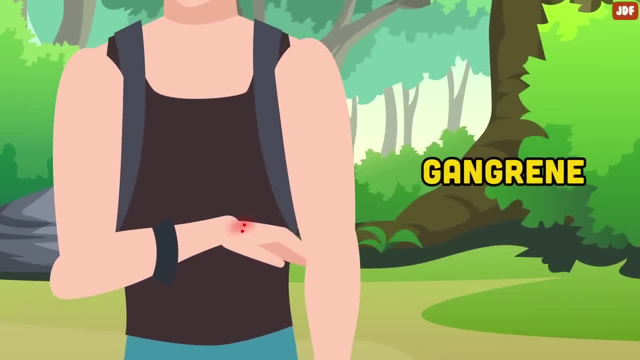 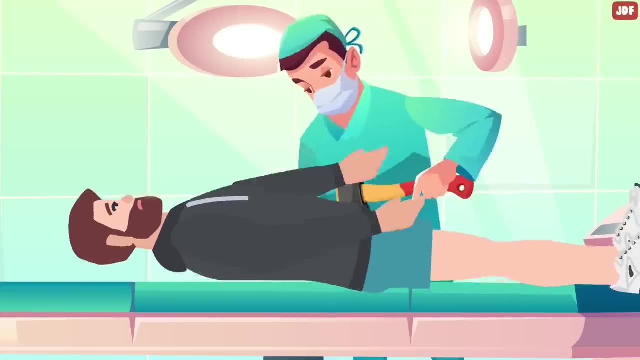 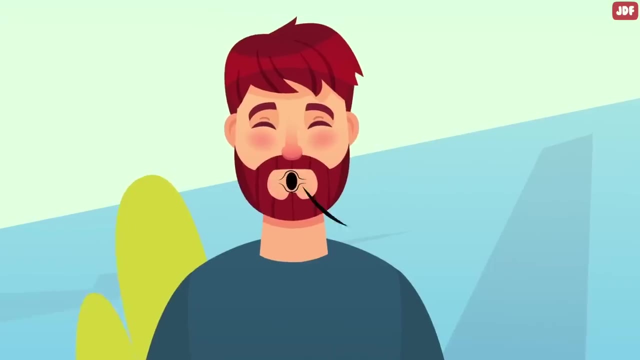 victim. Even worse, it increases the chance of gangrene, which means the concentrated venom near the bite will rapidly destroy cells. It usually ends with the victim losing a limb. Slashing the wound with a knife isn't going to help either. While it's easier said than done, staying calm and still after a snake bite will prevent your heart from 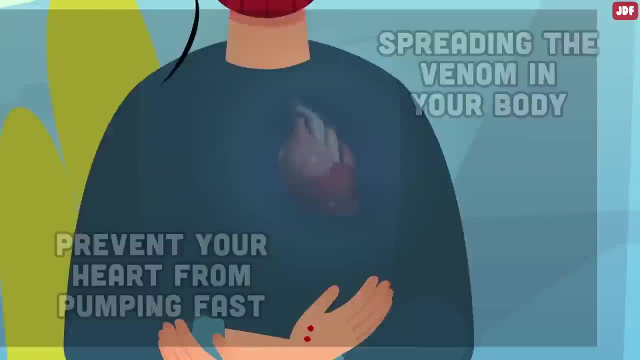 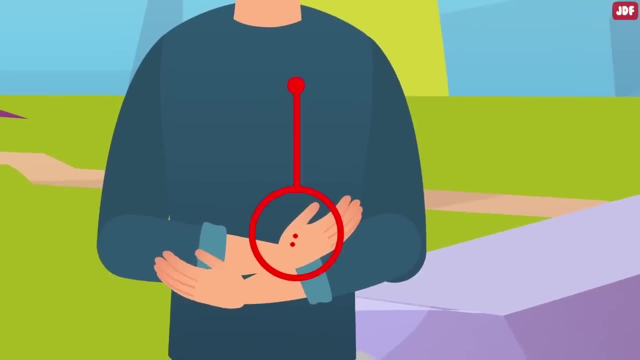 pumping fast and spreading the venom in your body. If you've been bitten by a poisonous snake, not moving might save your life. Lay or sit down with the bite below the level of the heart. wash the wound with warm soapy water and immediately call an emergency. 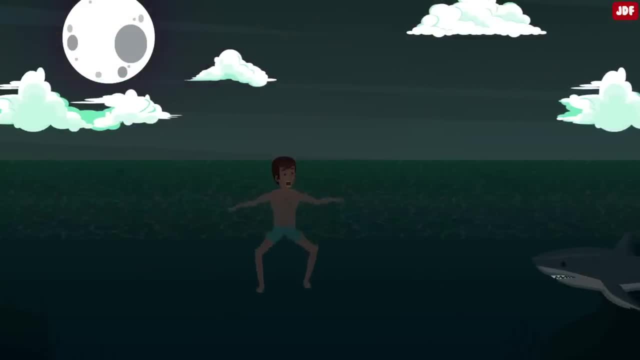 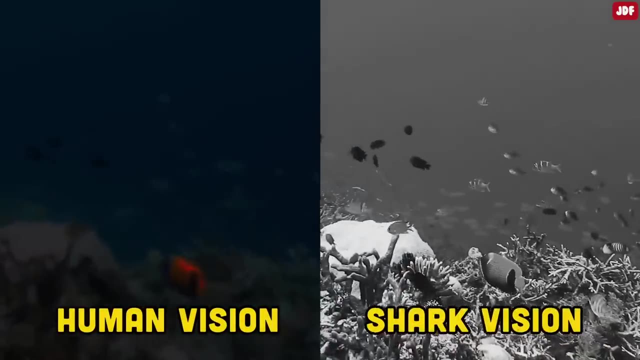 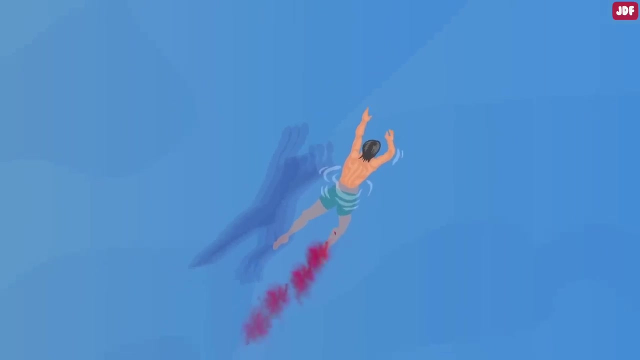 Sharks. To prevent a shark attack, scientists from the University of Florida recommend not swimming at dawn, dusk or night. Sharks are most active at these times and, unlike you, they are able to see in the dark. Don't allow blood to get into the water. Sharks can smell it from miles. 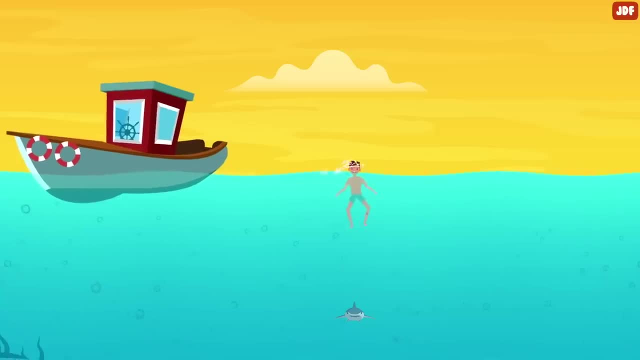 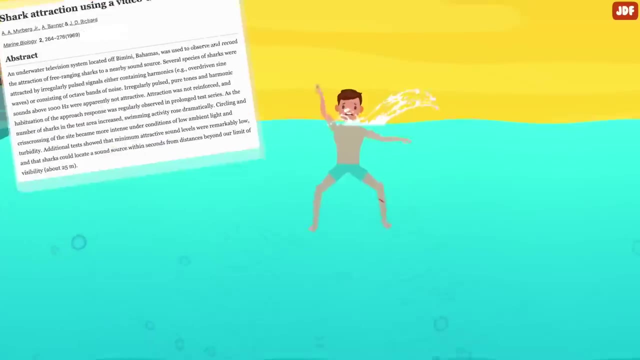 away If you're wounded, leave the water And remember not to make irregular sounds like those made by an injured fish swimming or splashing around. Research has shown that sound, rather than sight or smell, is a shark's primary cue for moving into an area. If you see a shark, 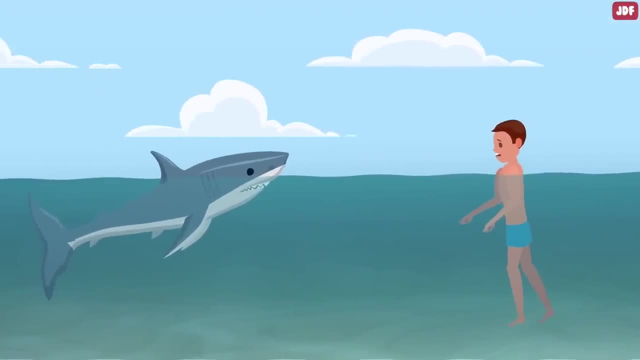 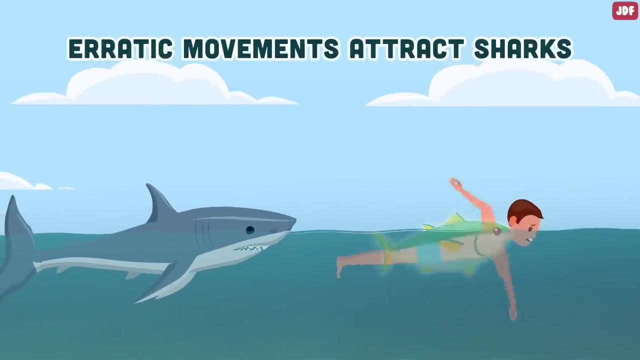 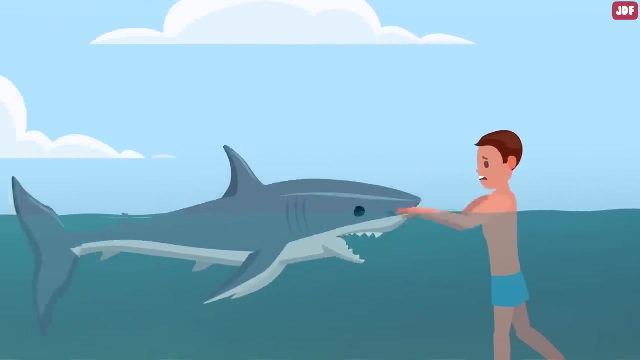 face-to-face but the shark is not attacking you. stay still, Don't make a splash and don't escape. You'll look like prey this way, and erratic movements attract sharks. Move very slowly and wait for the shark to swim away. If a shark is actively attacking, you claw. 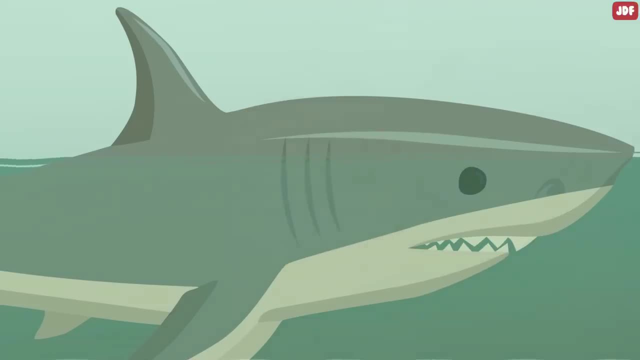 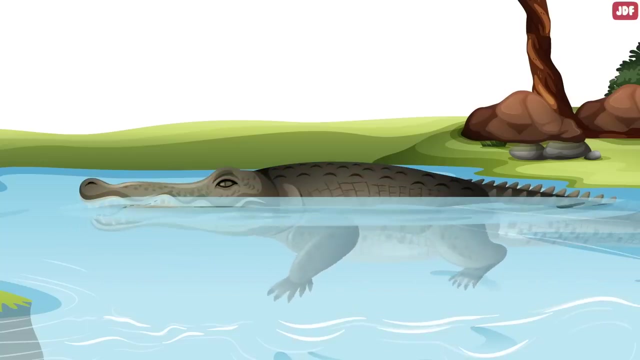 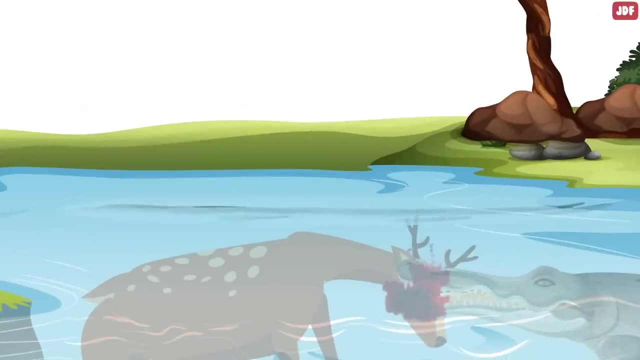 at its eyes and gills, as these zones are the most sensitive. Alligators or crocodiles. These animals prefer freshwater lakes and slow-moving rivers, and can hold their breath underwater for one to twenty-four hours. The jaws of these creatures are the strongest on the planet. so it's best to stay away from them. If you see a shark, don't make a splash and don't escape. Stay away from them. Don't make a splash and don't escape. Stay away from them, Don't escape. 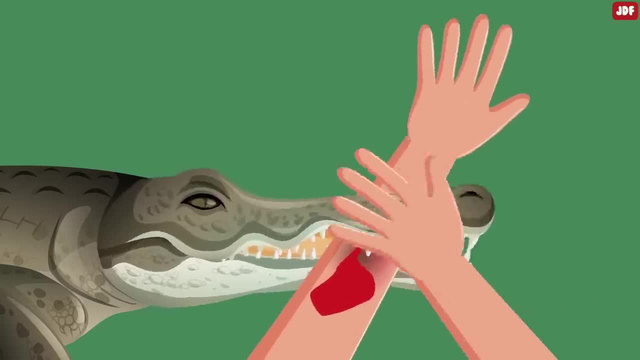 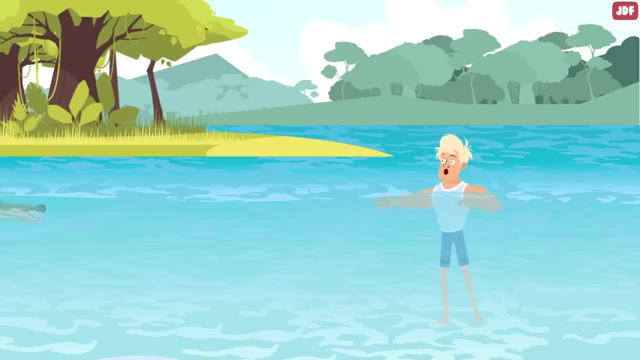 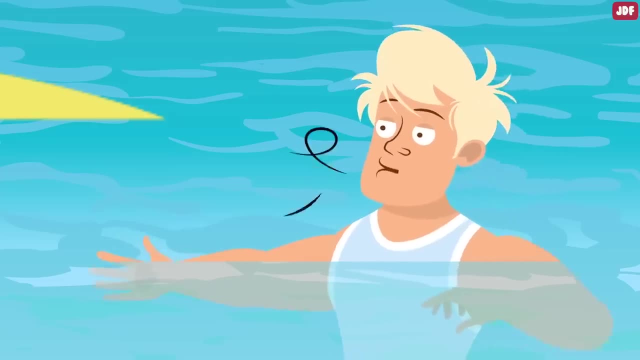 and can run up to eleven miles per hour. If you see a crocodile while swimming, don't make splashes and don't shout. It'll only draw attention. Try to be as calm as you can and quietly swim away. If a crocodile grabs you, hit its eyes. 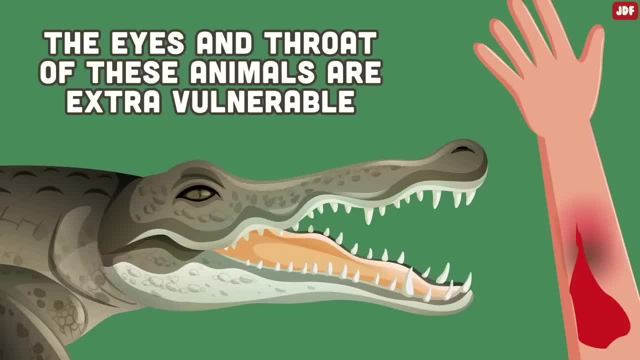 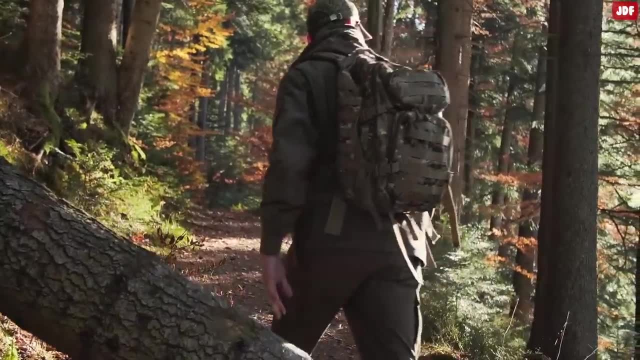 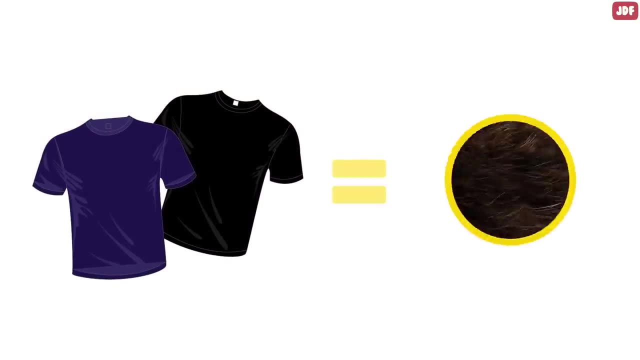 The eyes and throat of these animals are extra vulnerable and definitely don't play dead Bees. When hiking in the wilderness, where there are going to be bees, wear light-colored clothing. Dark-colored clothing appears more threatening to bees. This is because dark clothes resemble the fur of their natural predators. 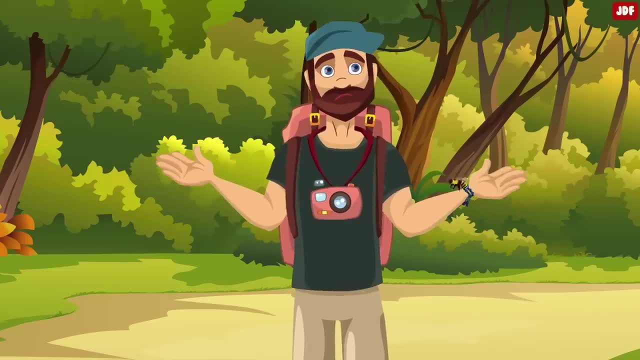 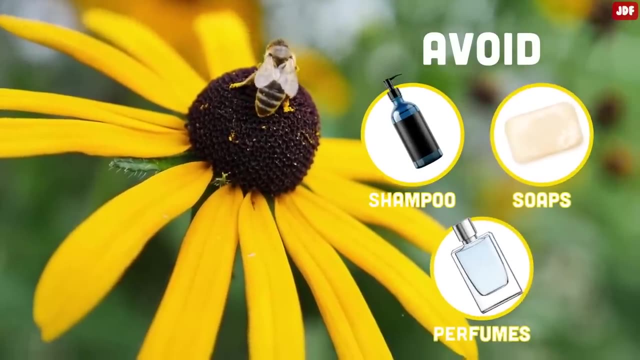 like bears and skunks. So if you wear a black shirt, your chances of getting stung are higher, And try to avoid strongly-scented shampoo, soaps and perfumes. According to Japanese scientists from Tamagawa University, perfume has scent that. 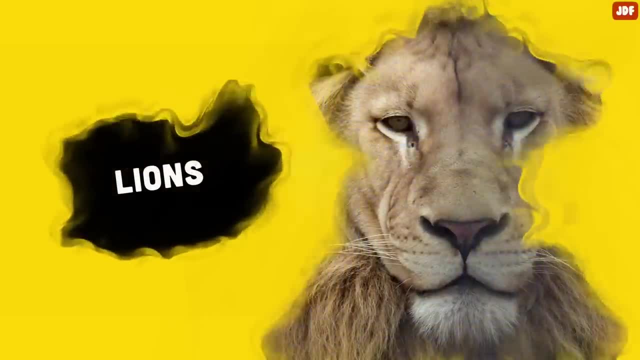 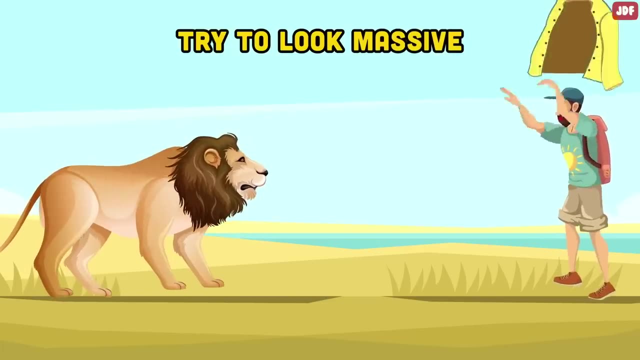 angers bees, Lions. If you have encountered a lion, maintain eye contact and don't run. Try to look massive by raising your arms and opening your jacket. Doing this will make a lion think that you are stronger than it. Slowly wave your arms, speak firmly and throw items at the lion if necessary. 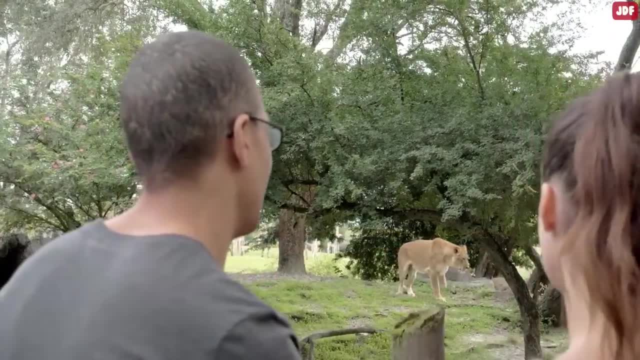 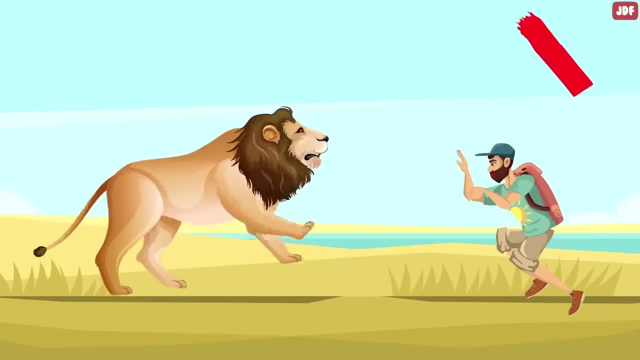 Normally the lion will move on. You should be confident when facing a lion so the animal perceives your presence threatening and avoid the encounter. Never crouch down or bend over. Biologists surmise lions don't recognize standing humans as prey. 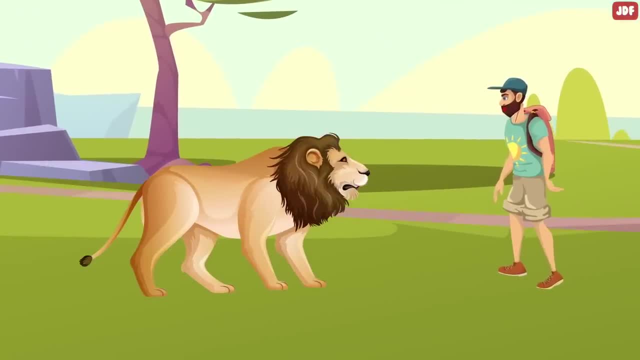 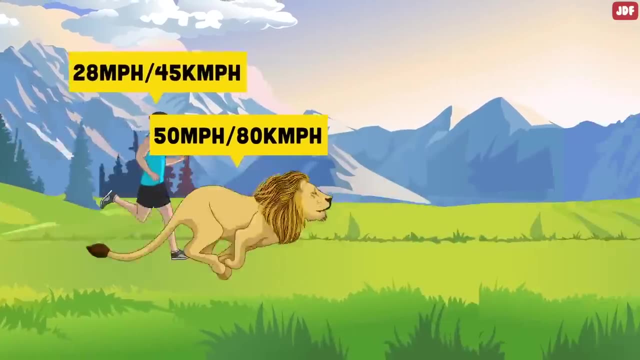 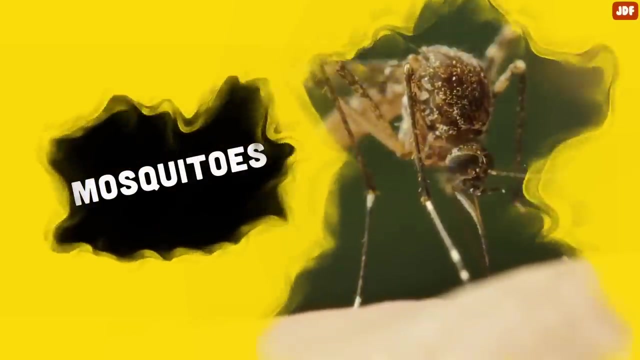 Should the lion charge you, you still must not run. This will obviously be difficult. It should not surprise you that a lion is way faster than you, and lions like to attack from behind. Most charges are mock charges, so stay still. Mosquitoes: Research has shown that mosquitoes are attracted to the color black. 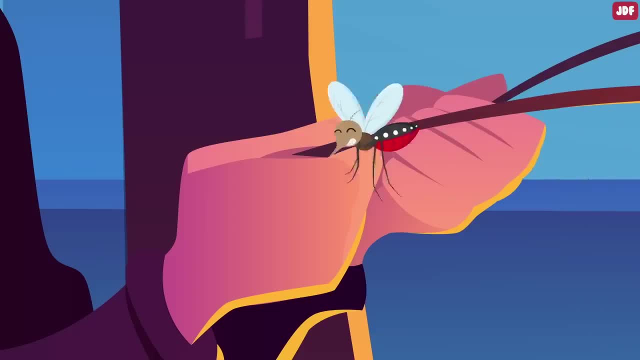 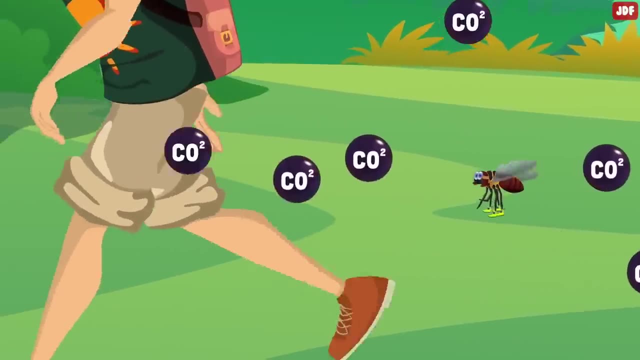 If you're wearing dark colors, your chances of being stung by these insects are much higher. Apart from vision, mosquitoes locate us by tracking down the carbon dioxide we emit As we exercise and exhale more excessively. our body gives off more heat- sweat. 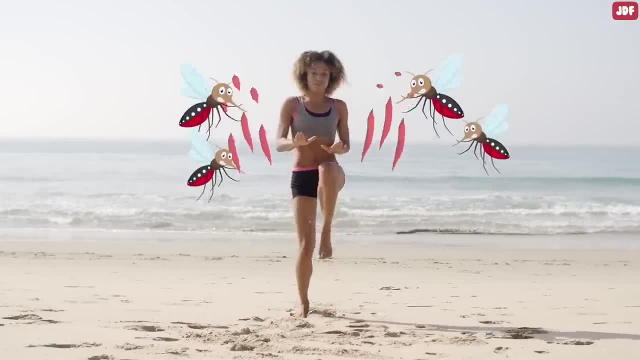 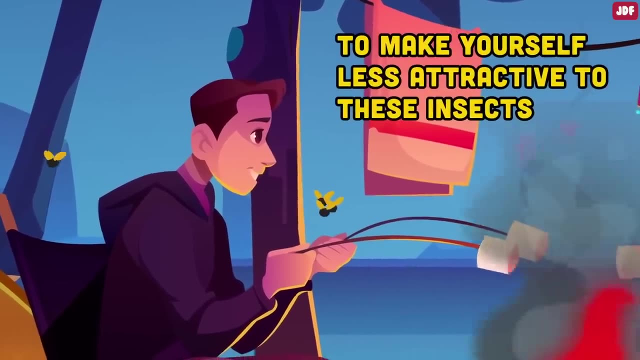 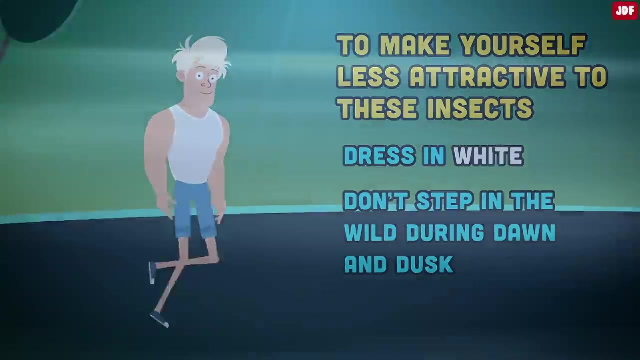 and carbon dioxide, which attracts more mosquitoes. Mosquitoes prefer cooler and shaded areas as opposed to direct sunlight. So to make yourself less attractive to these insects, dress in white and don't step in the wild during the day. If you're wearing dark colors, dress in white and don't step in the wild during the day. 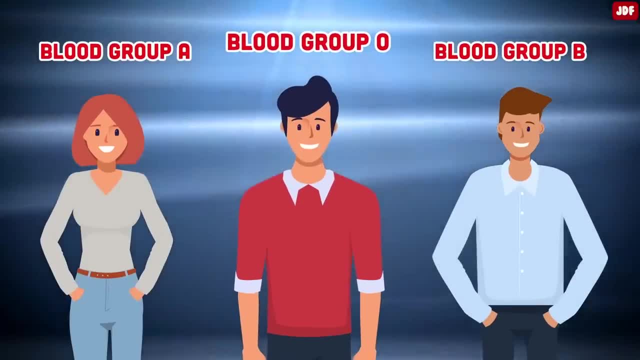 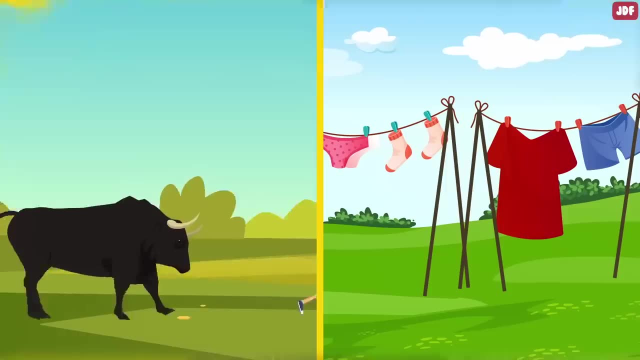 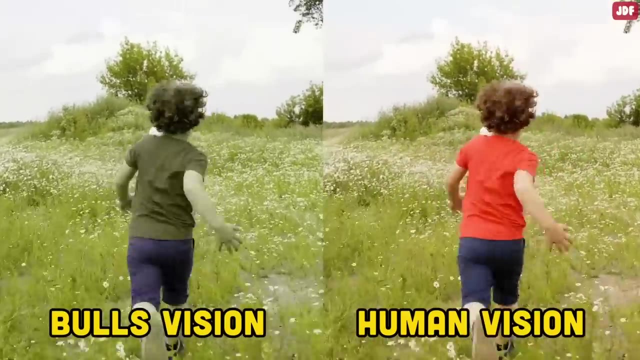 And remember: many studies have shown that those with blood type O are almost twice as attractive to mosquitoes Bulls. Opposite to the common misconception, bulls react to movements and not to the red color. In fact, bulls are colorblind and can't distinguish the red color. 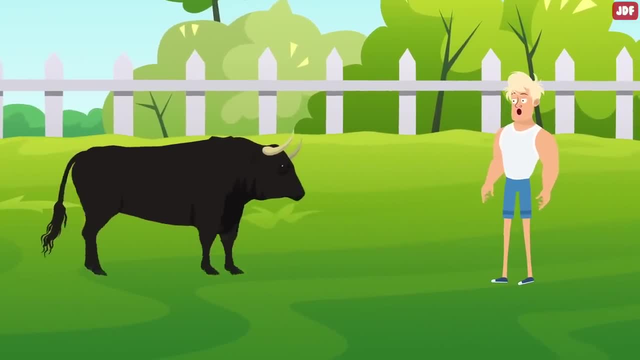 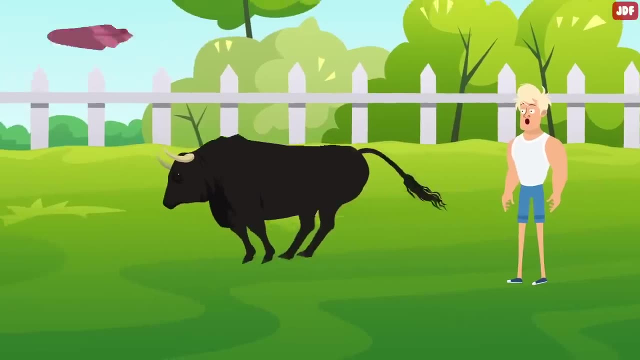 So if a bull is running at you, stand still and straight. Use your jacket, t-shirt or other clothes that are comfortable to wear, like yourilles orństh photographer, and step in the water early. The animal will change direction and follow that object. Jellyfish Sting so that they can catch and eat other sea creatures, But that sting can be turned on you if you brush against them while swimming in the ocean. Some people believe that peeing on the bitten zone can relieve the pain, But it's just a myth. 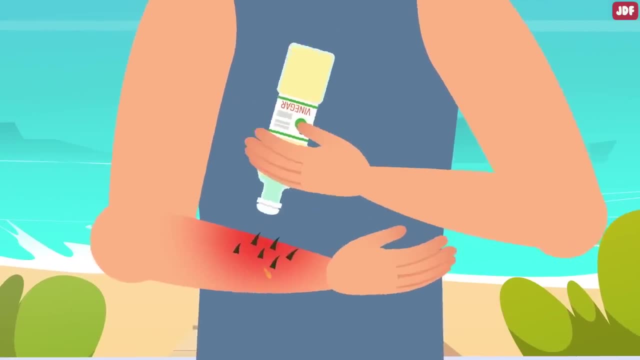 If you do find yourself with a jellyfish burn, rinse the area with vinegar or soak the skin in hot water. After that, use tweezers to pull off any tentacles still on your skin. Elephant Attack. Elephants are friendly and intelligent. 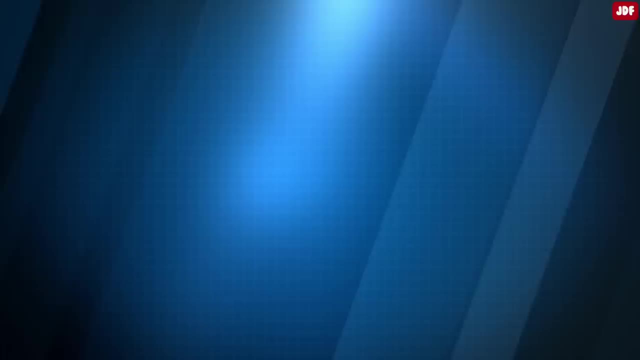 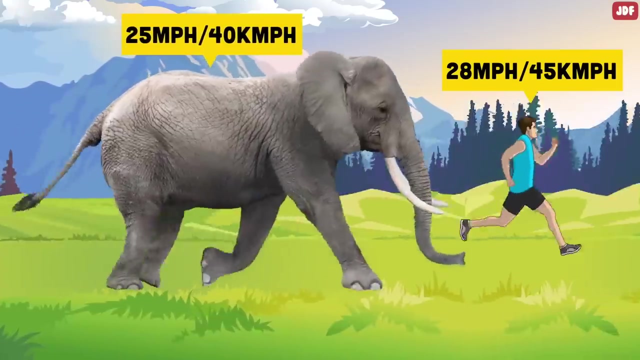 animals, but they are known to attack people. It's especially true about female elephant mothers, who perceive you as a threat to their babies. Since elephants can run up to 25 miles an hour, you have little chance about running them. If you come across an elephant, it's best to read their body. 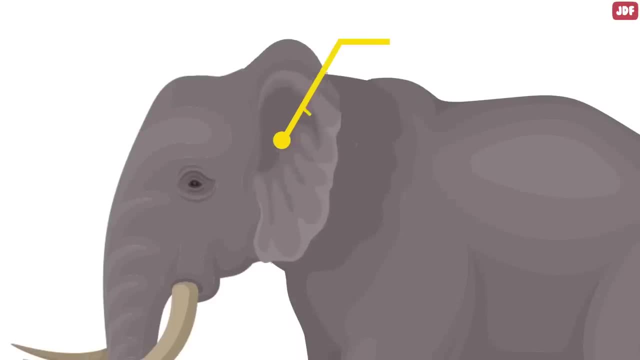 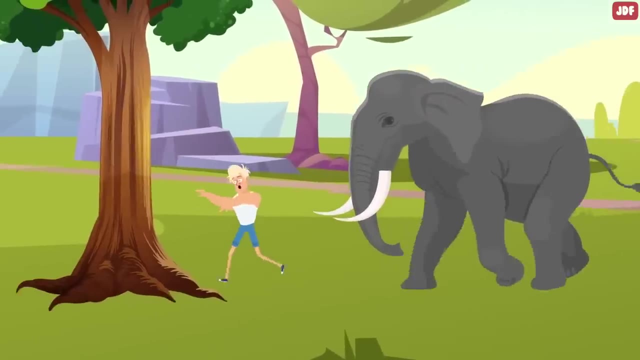 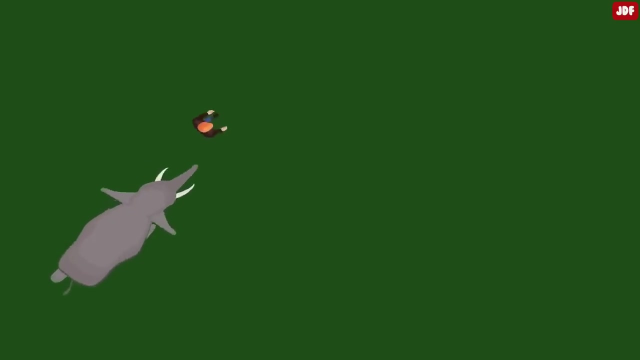 language and get signals early. If their ears are pinned back and the trunk is curved inwardly, it means they are going to attack you. If you're on foot, try to find a barrier between you and the elephant. This could be a big tree, vehicle or building. If there is no barrier around, 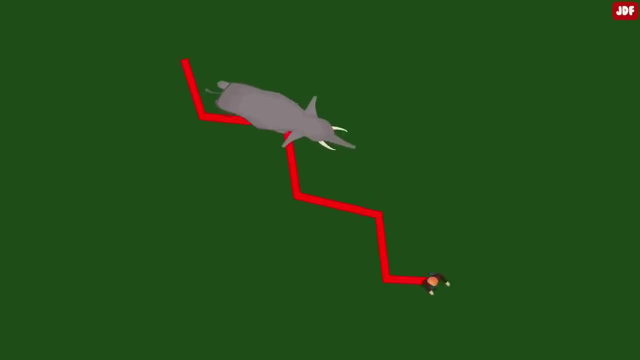 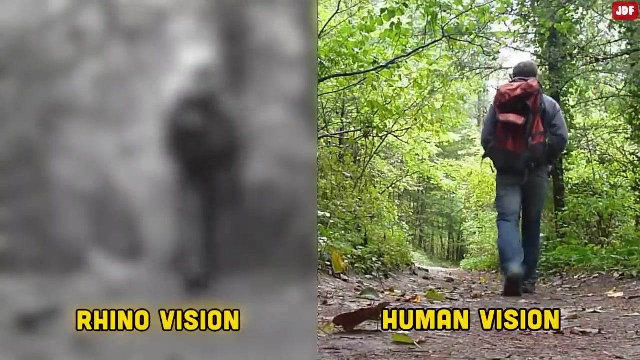 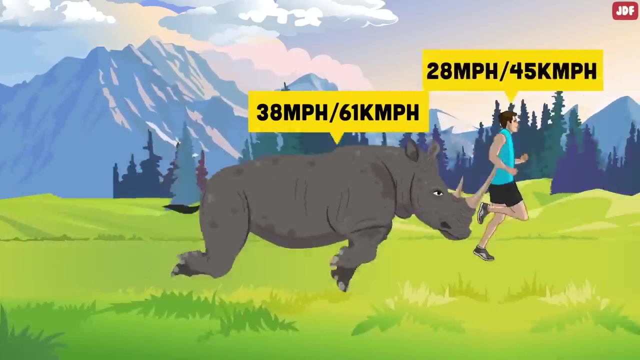 run in a zigzag pattern. It's difficult for elephants to change directions because of their heavy size. Rhinos- Rhinos' eyesight is one of the worst in the animal kingdom. Up there, with bulls and bats, Their speed can reach 38 miles per hour, which is why it's hard.